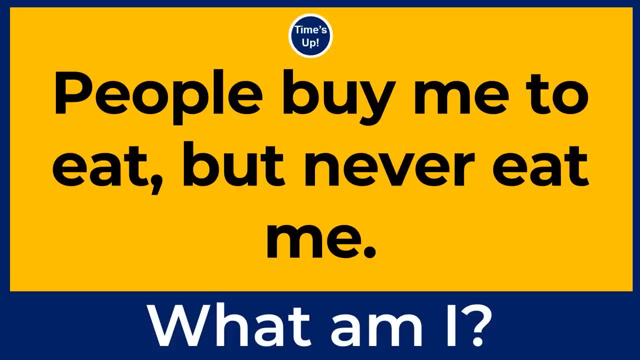 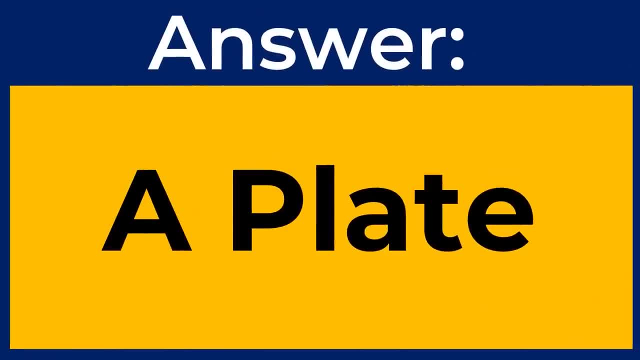 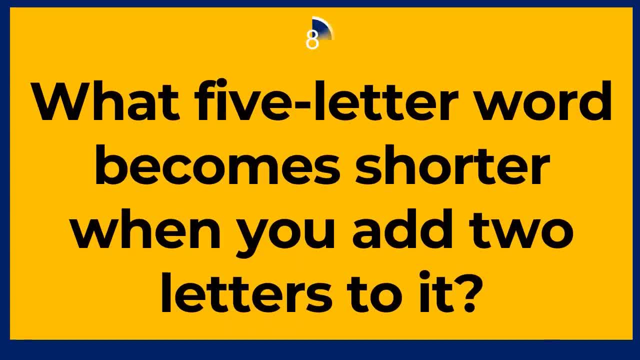 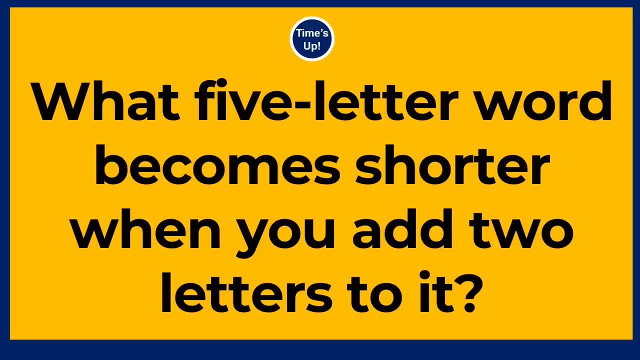 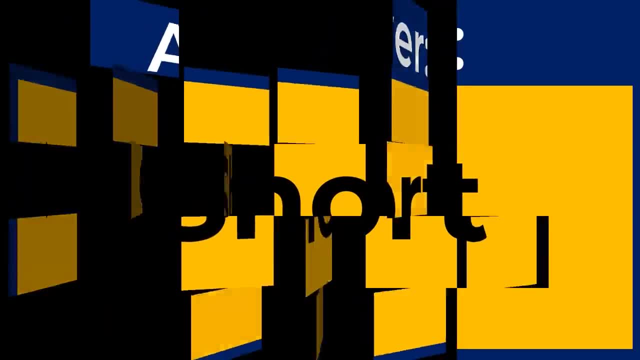 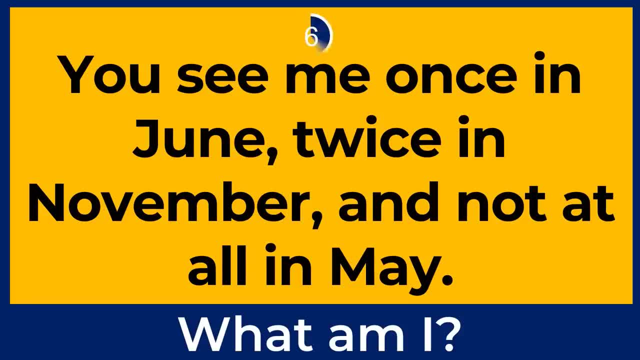 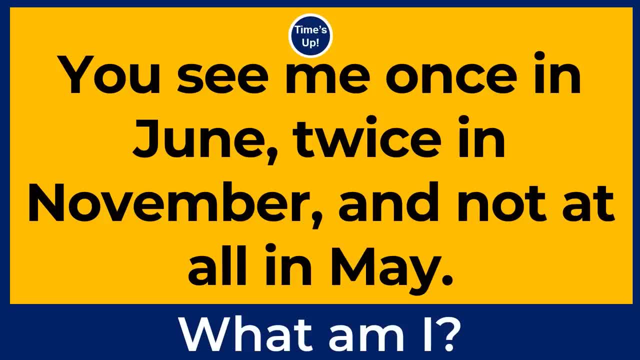 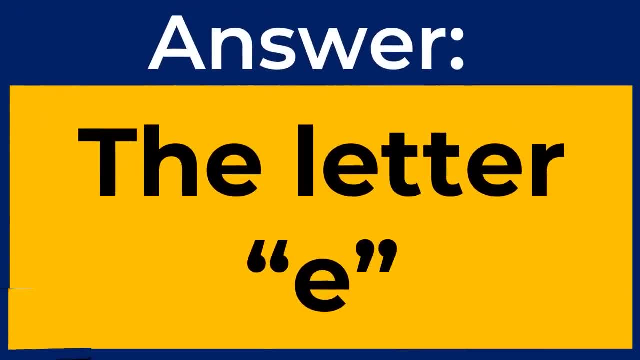 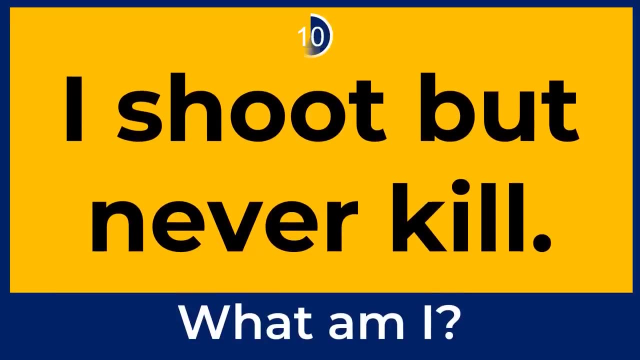 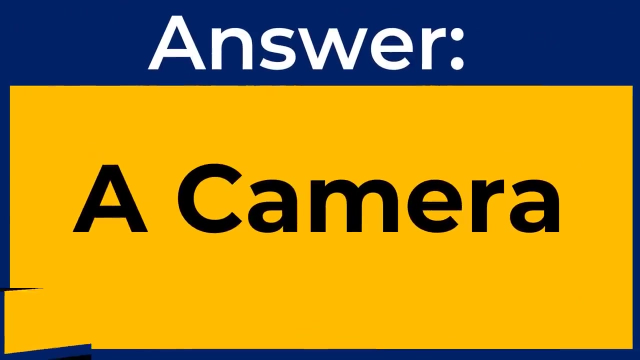 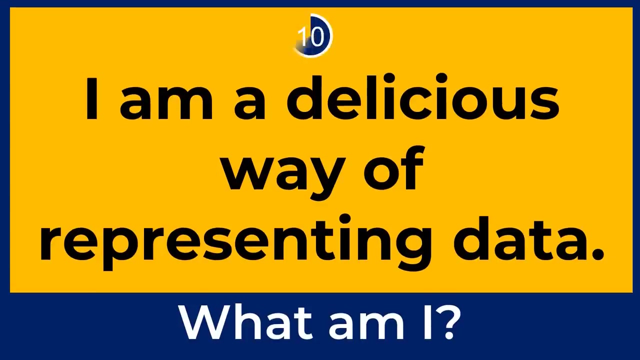 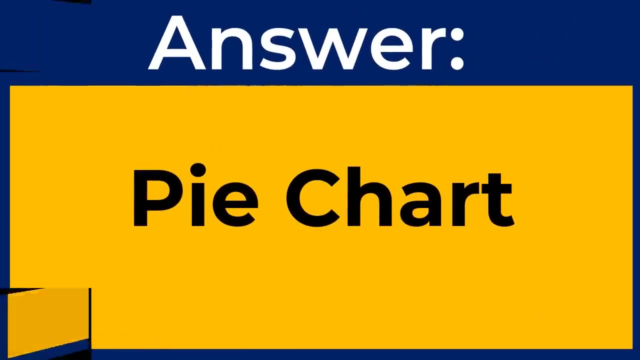 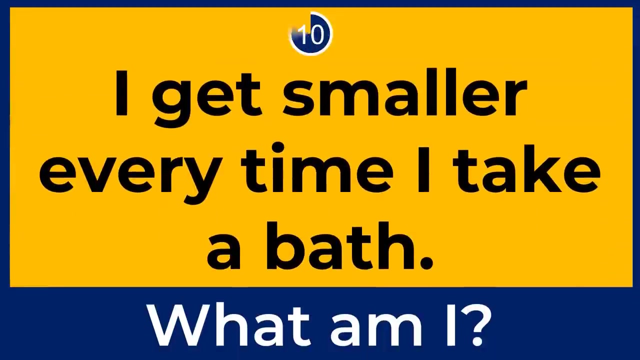 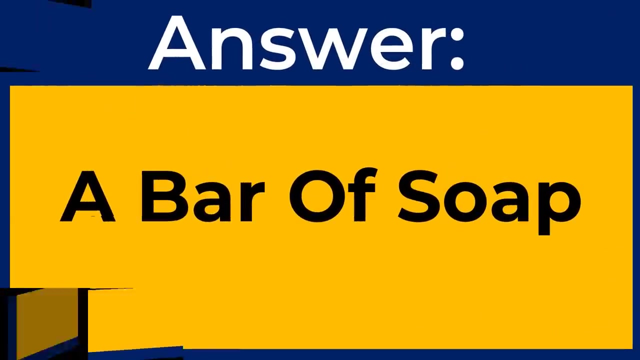 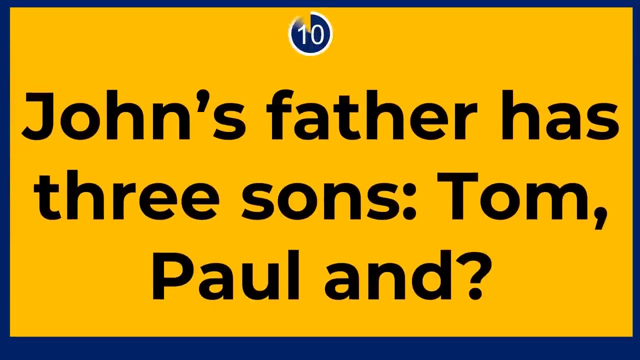 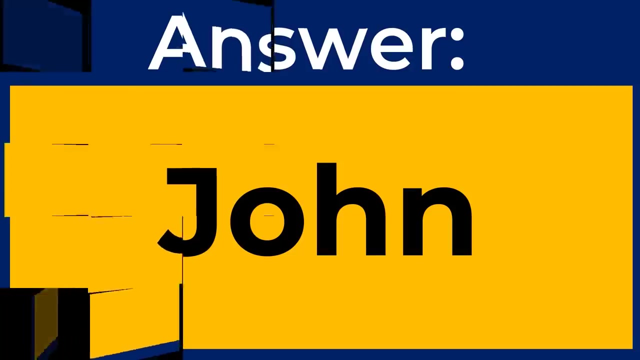 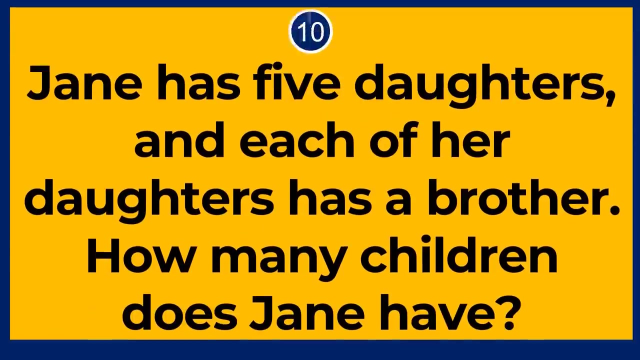 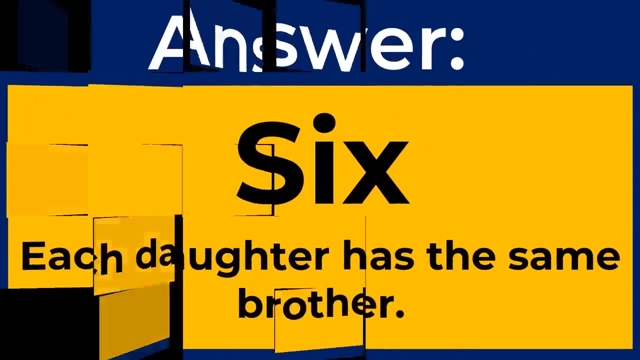 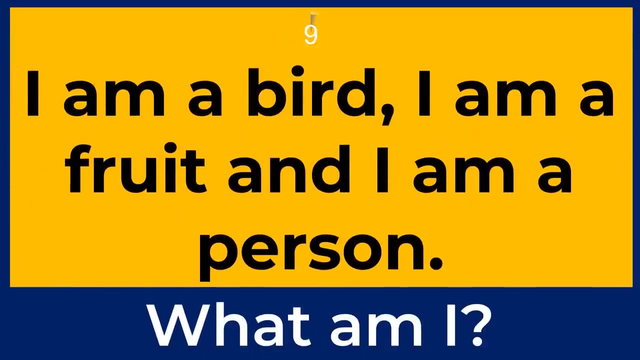 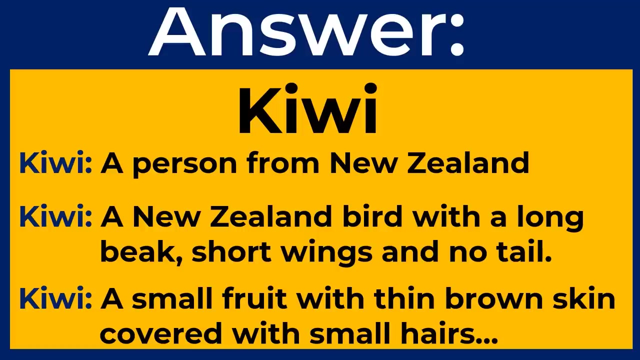 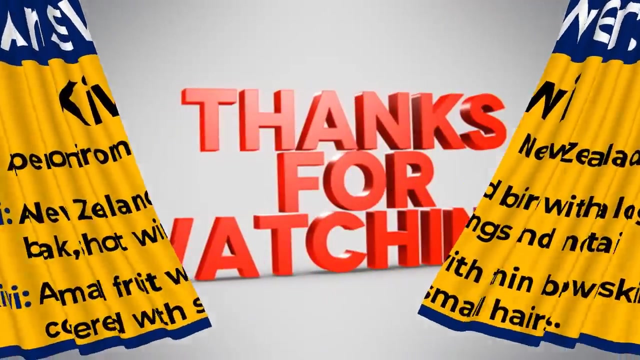 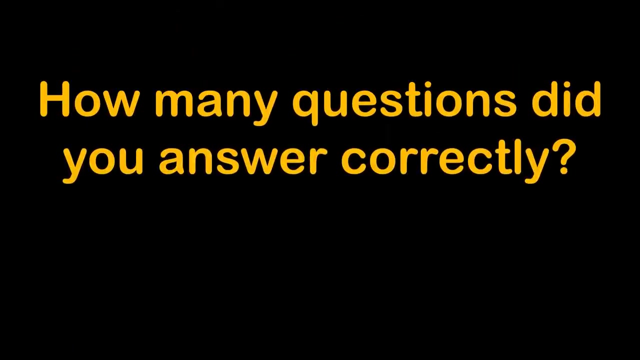 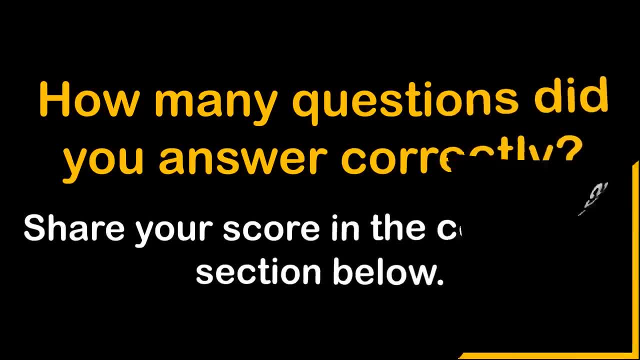 Share your score in the comment section below. Subscribe. Please share with your friends.